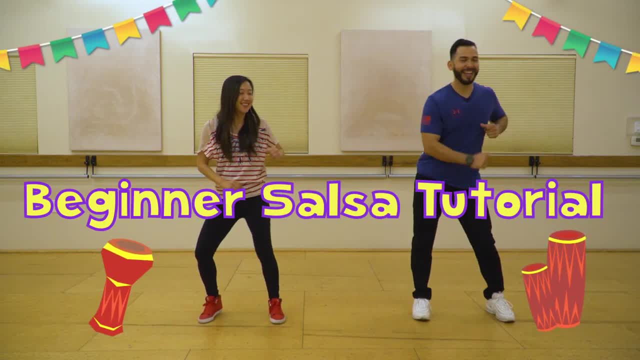 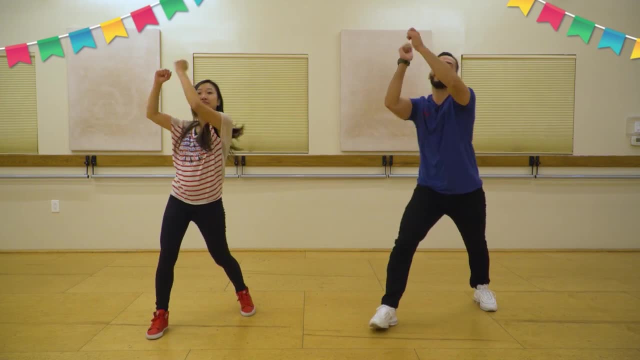 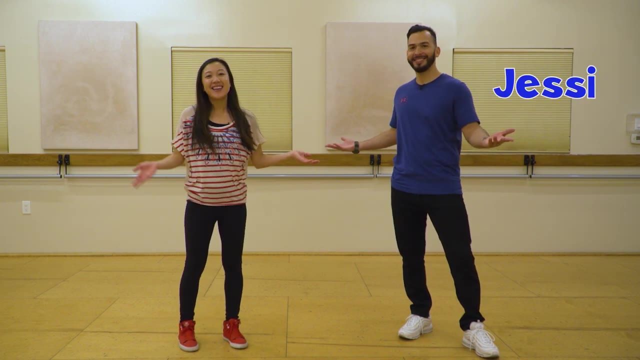 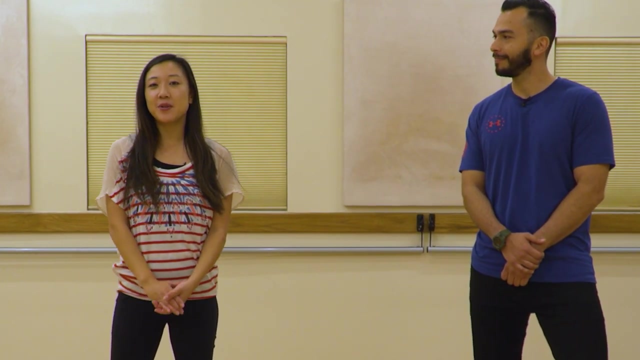 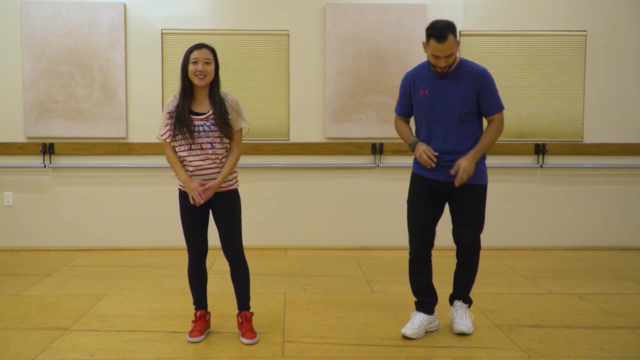 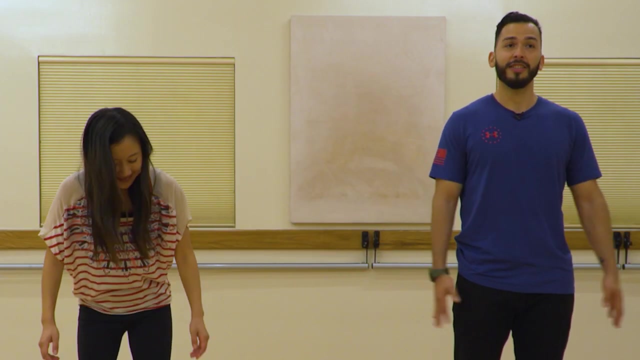 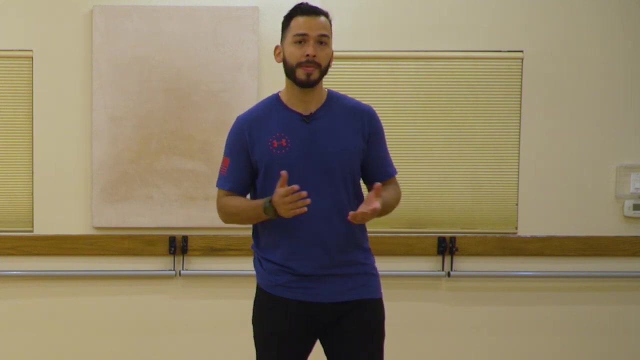 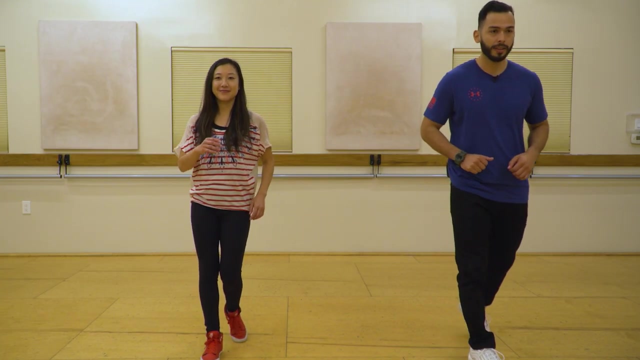 Hi guys, this is Noah and Jesse, Hey, and we're going to teach a salsa tutorial, a basic salsa class for you, where we'll break down a couple of basic moves. Feel free to grab your shoes or socks, because we're going to get right into it. So take it away, Jesse. First of all, let's all shake it off. Okay, so salsa is all about having fun. So this is what we're going to do. We're going to start off with the basic on one, So it's going to be three steps starting, So you can start with your left foot. We're going to go left, right, left. One more time. We're going left. 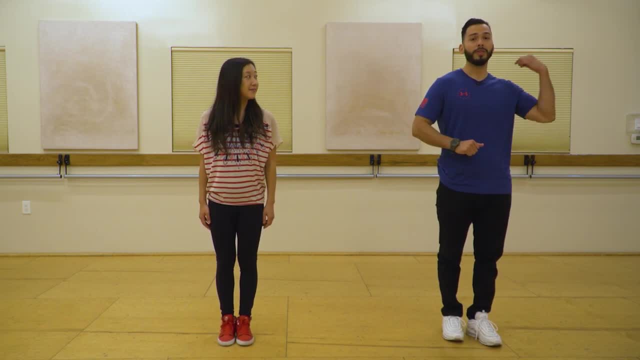 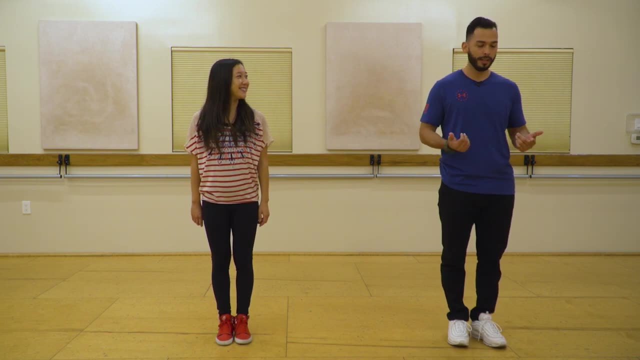 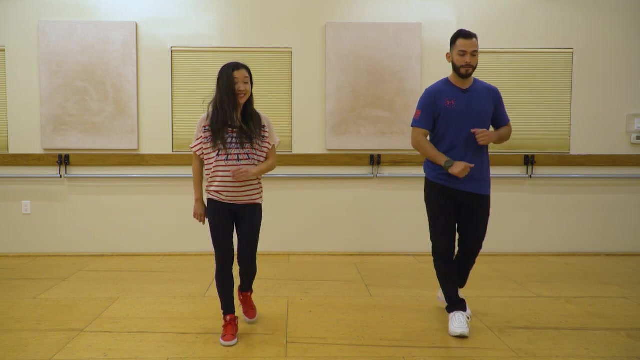 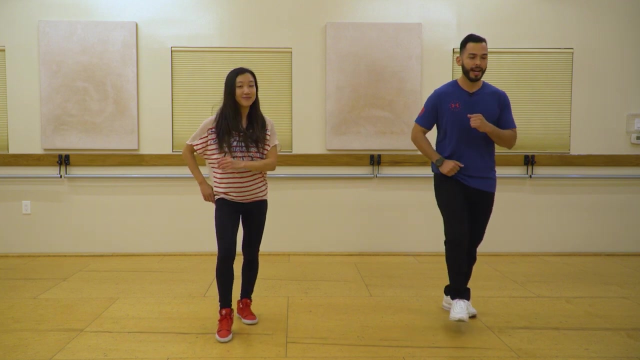 right, left. Now we're going to sit back with our right foot Ready. One, two, three, right, left, right, So all together Five, six, seven, eight. We're going: one, two, three, five, six, seven. One more time: We're going: one, two, three, five, six, seven. Here's a tip. Think about a refrigerated door. You're going to. 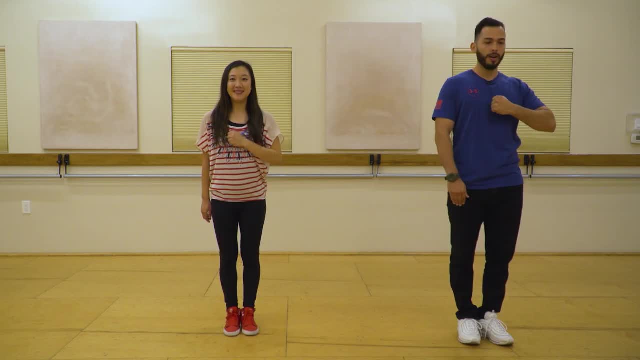 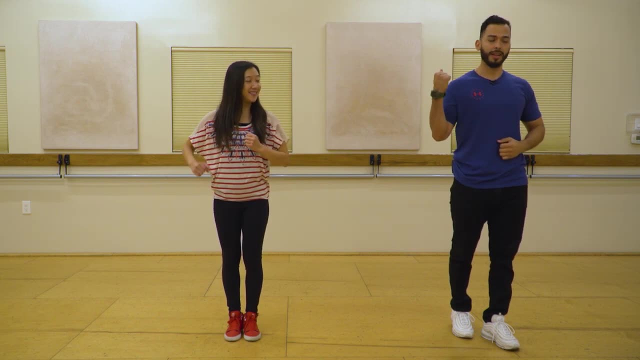 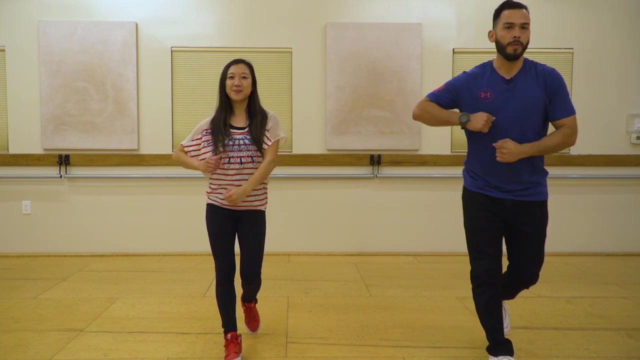 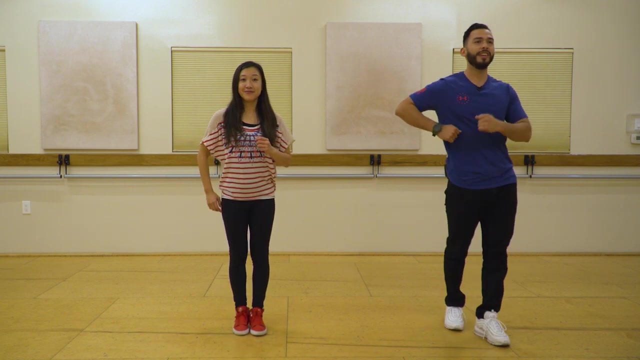 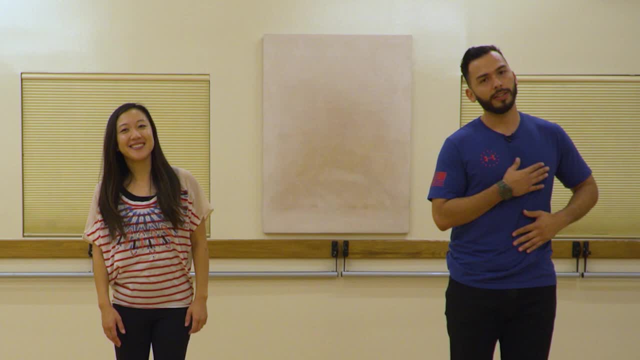 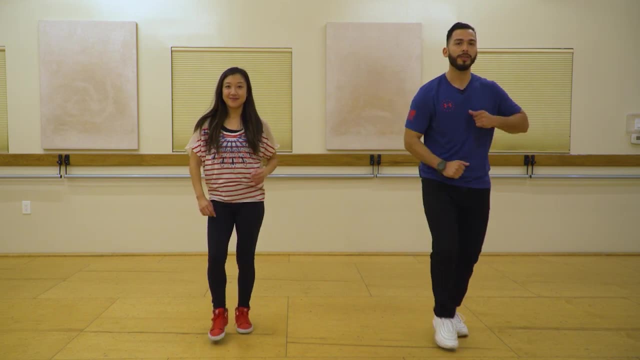 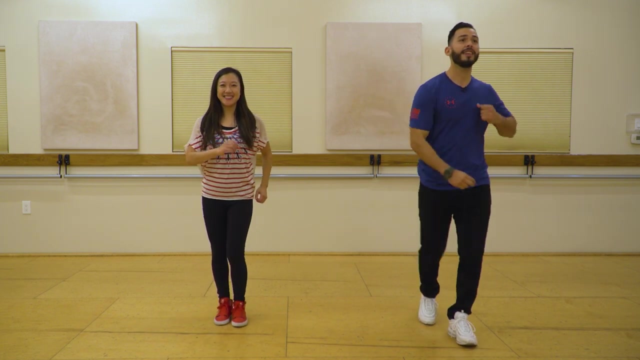 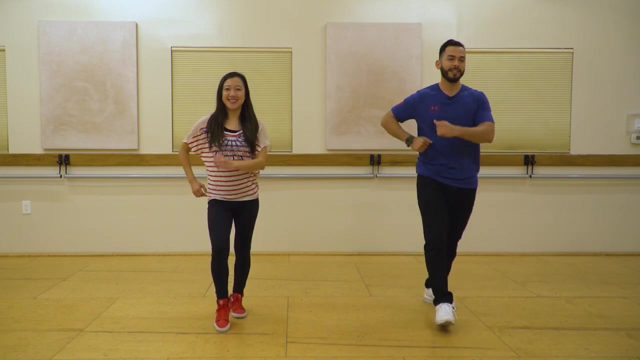 from right to left, left to right, left to right. So let's do it one more time. Let's do it again: Five, six, seven, eight. One, two, three, five, six, seven. One, two, three, five, six, seven. One, two, three, five, six, seven And a one, two, three, five, six, seven. How do you guys feel? Wow, That was so great. 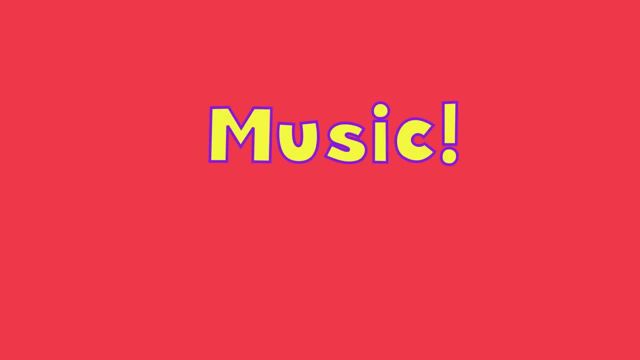 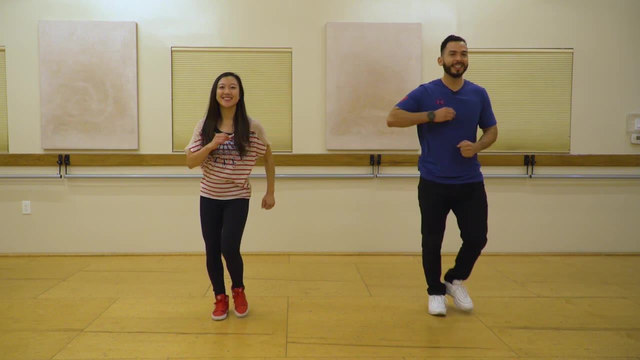 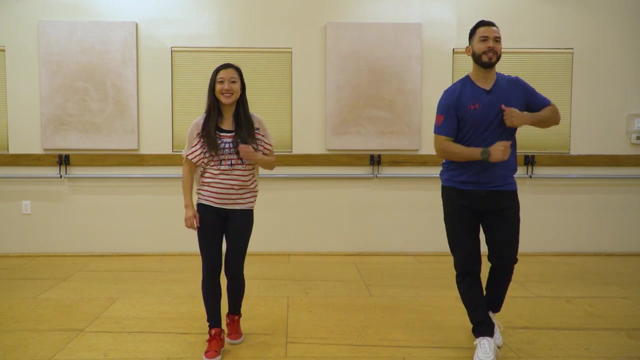 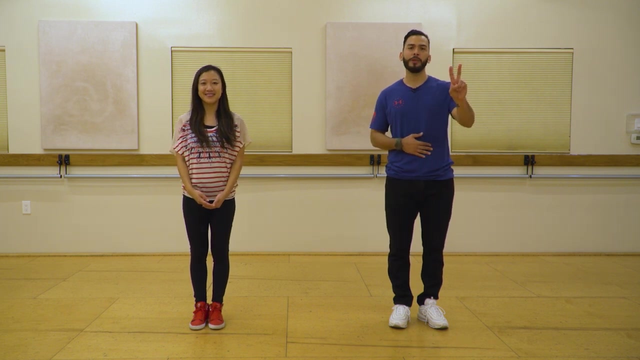 Let's try it with music. Yes, let's do it Ready. Five, six seven, eight. One, two, three, five, six, seven, One, two, three, five, six, seven, One, two, three, five, six, seven. One, two, three and five six seven. Nice, Good job. So we're going to do our second basic move, And this is from left to right, right to left, And this is how it goes. We're doing the 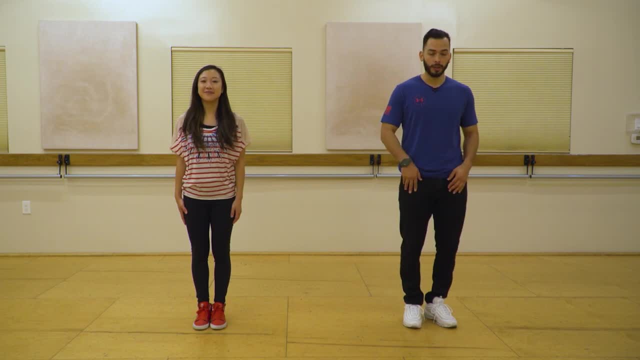 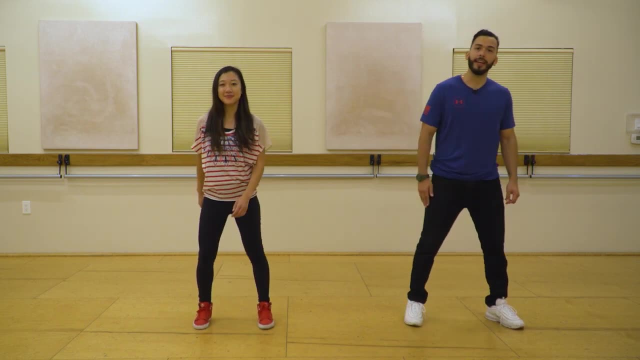 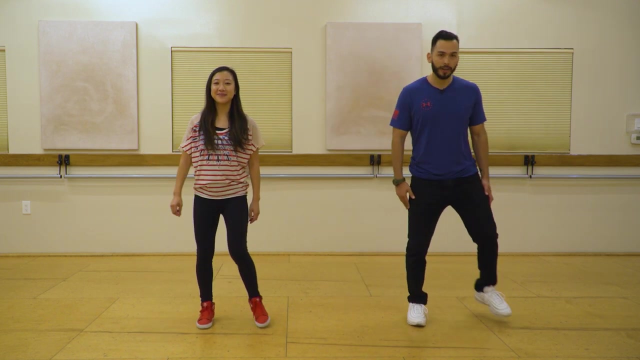 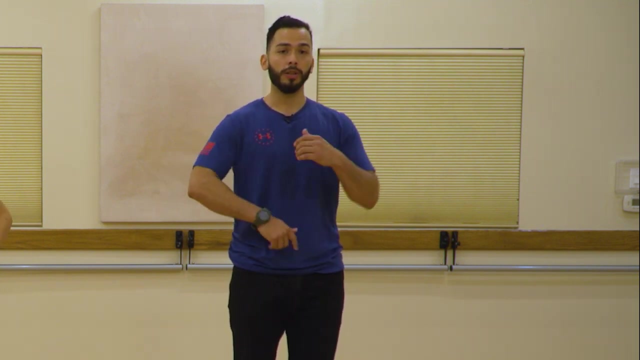 same steps, with the left foot starting out first. We're going left, right, left, Now to the right, right, left, right. One more time, Left, right, left, right, foot right. Good, Now, don't forget, we have our hands up here, So we always want to move where we're going right, So let's do it, Thinking about it centered. We're going to go five, six, seven, eight. 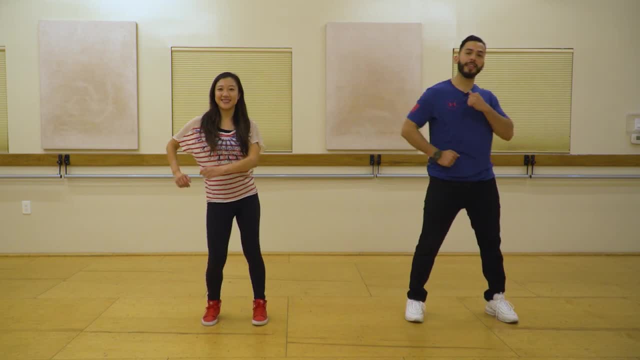 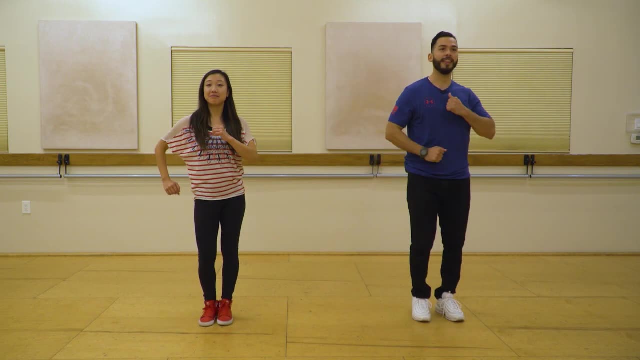 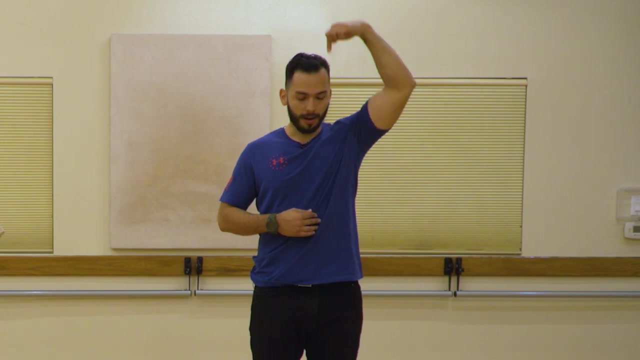 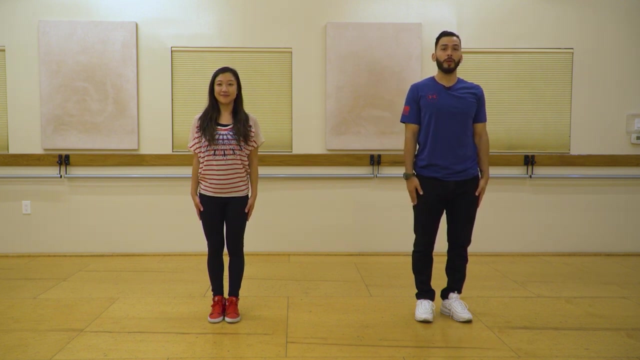 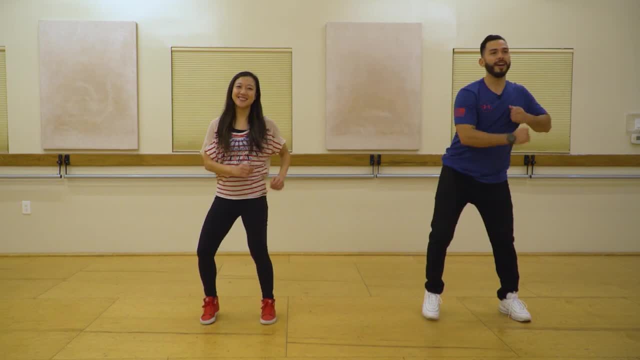 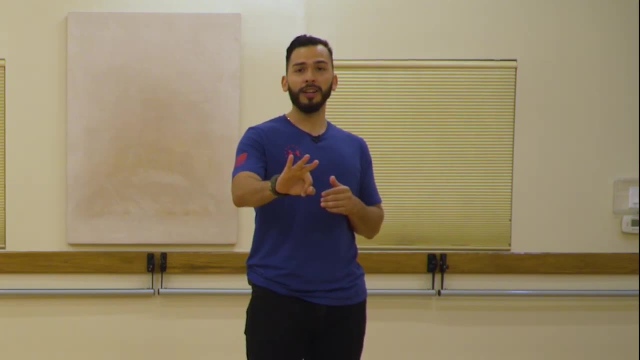 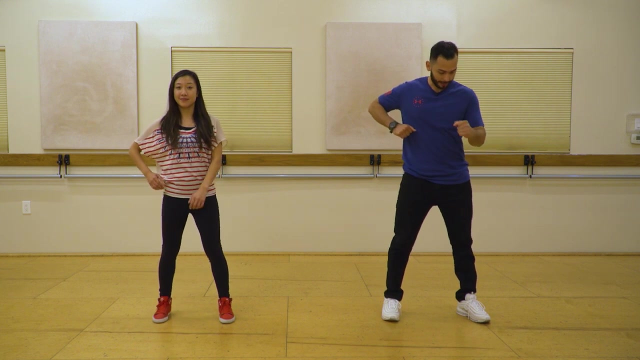 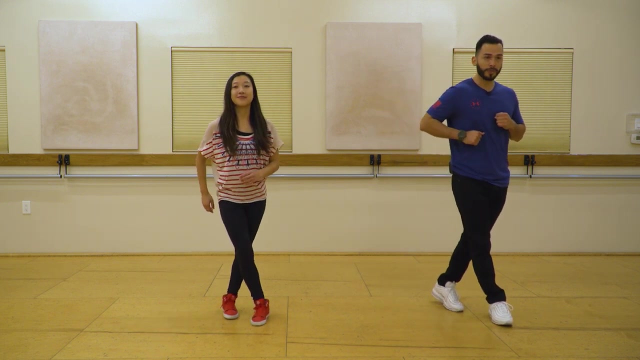 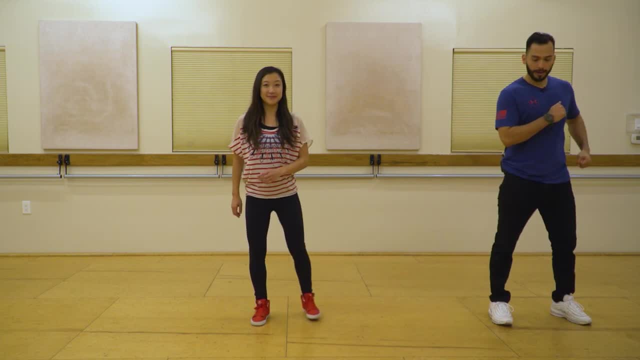 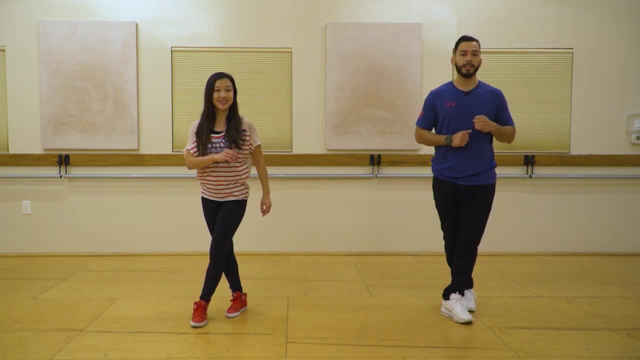 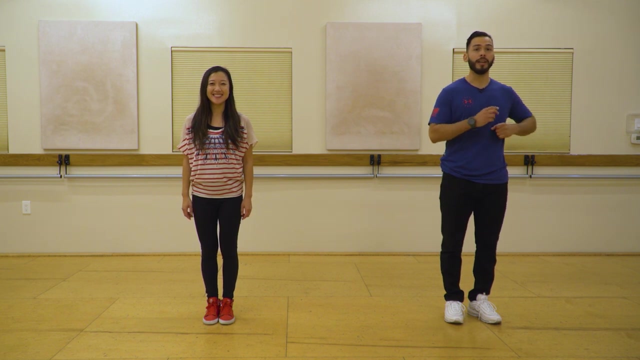 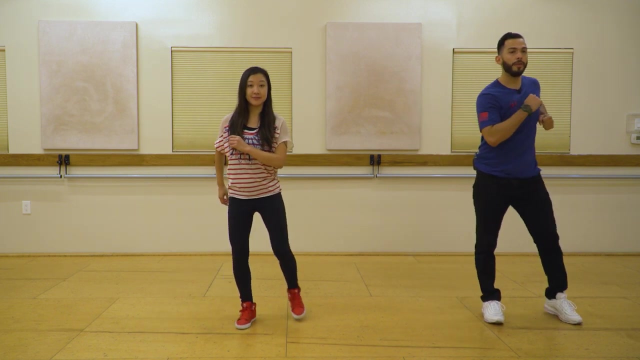 finish it off to the right foot. going to the right, right, move your left foot just a little bit back left and then your right foot crosses, Boom, Nice. So let's start from the beginning again. It's a little complicated, but you got it. You guys got this Ready. One more time You're going left, right foot back, boom, and then left, boom. Now right foot out right, left foot back, left, boom, Nice. Now let's do. 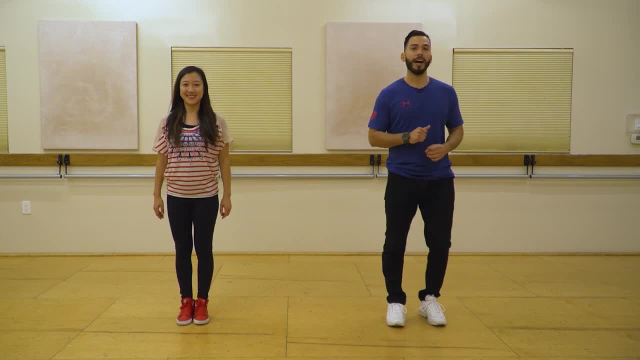 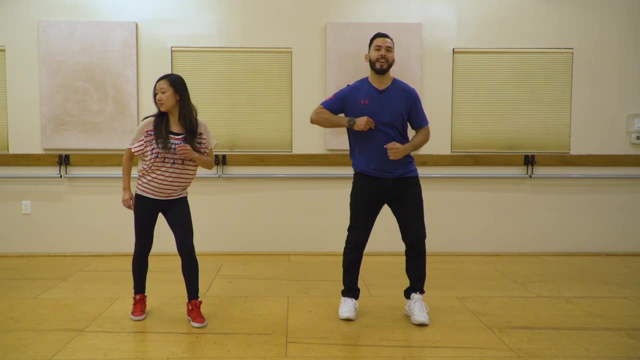 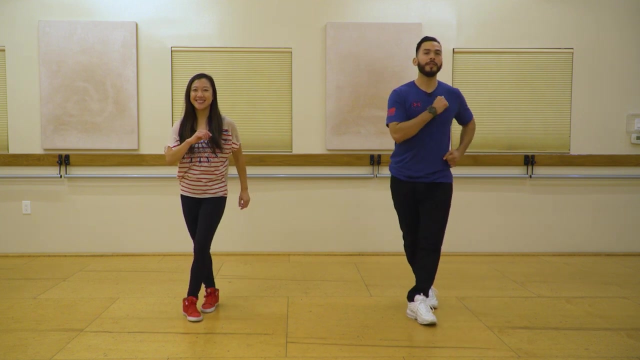 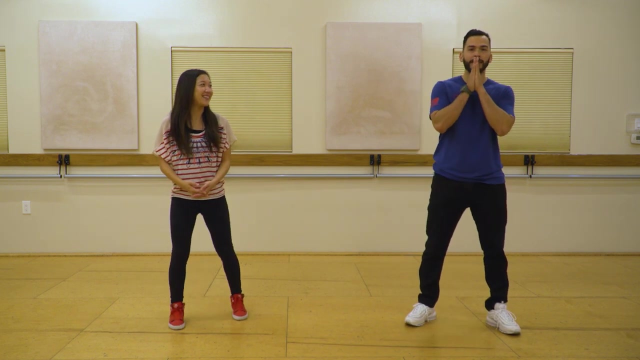 it all together Ready, Five, six, five, six, seven, eight. Left right, left right, foot right, left right, left right, foot right. One more time: Left right, left, right, foot left, left right, left right, foot right. Good job, Music, Music, Let's do it. Five, six, seven, eight. 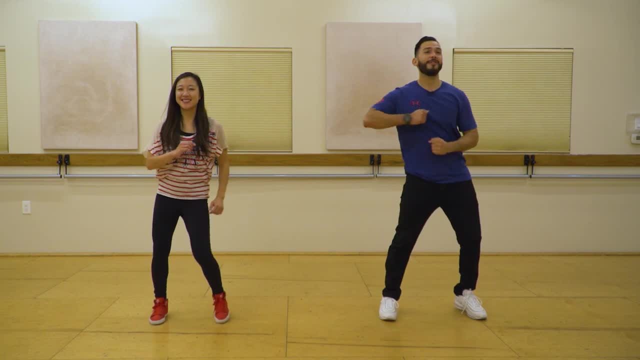 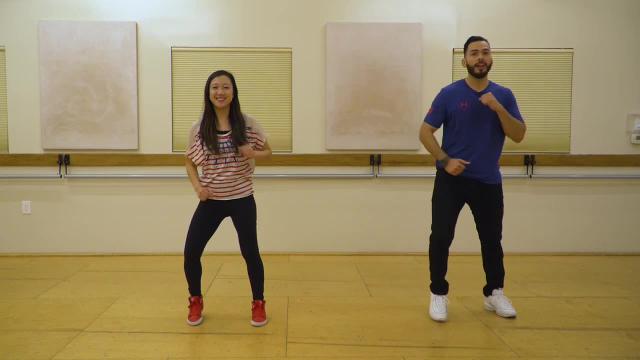 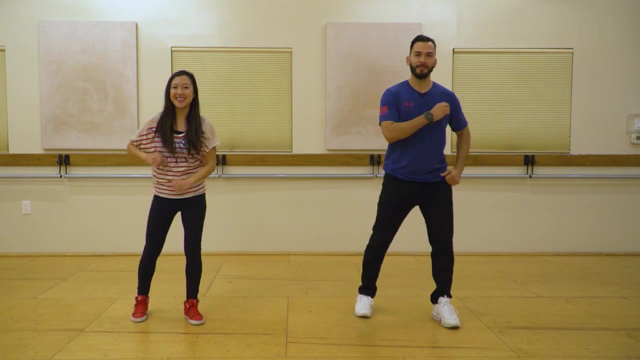 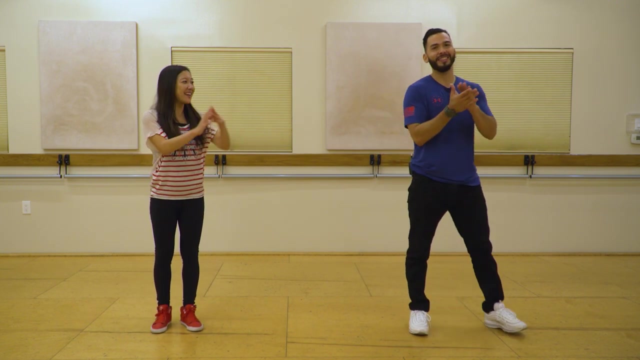 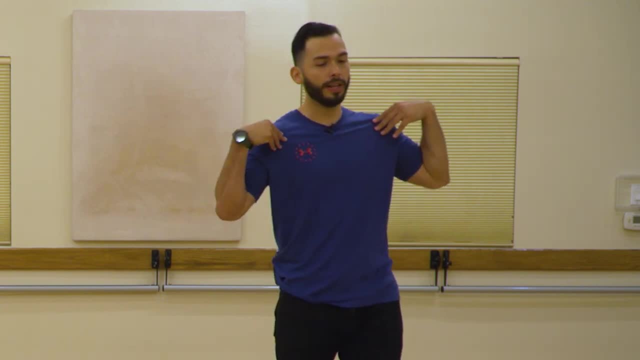 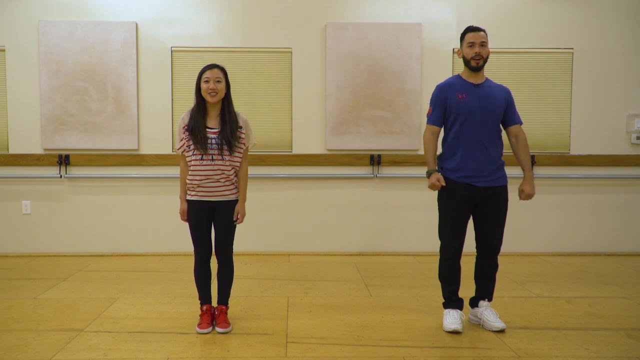 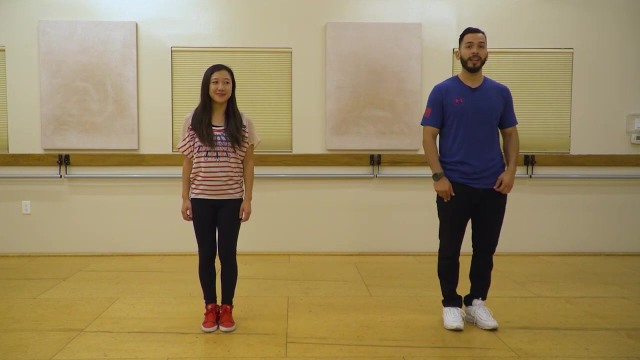 Now we're going to move a little bit of our upper body. So here we go To the same side, to the left. we're going to start out. We're going to use our shoulders, right, It's going to be a little shimmy, So just shake it off. Can I show you where your shoulders are Right here We're going to shake it off. okay, So we're going to do the same steps that we did for the side basic. We're going to go left, right, left right, left right. But now we're going to use our shoulders Ready, Five, six, seven, eight. Shake it off, Shake it off And we're going to go left right, left right, left right. 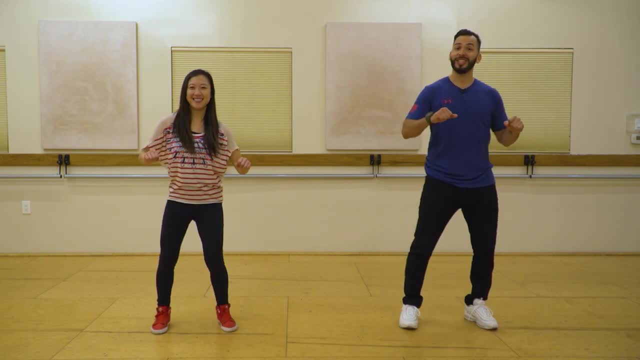 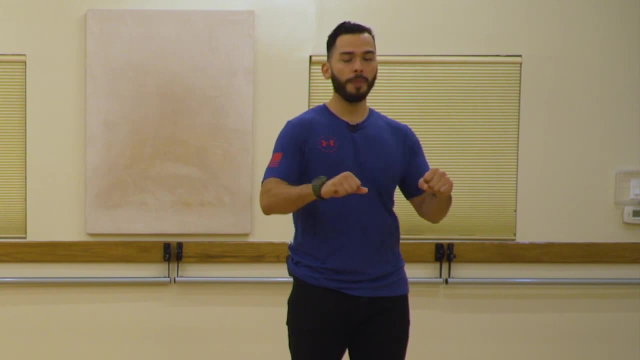 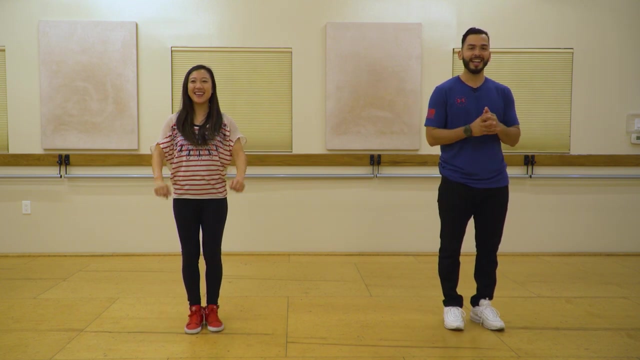 time. Shake it off, shake it off, shake it off and shake it off, Nice. So just remember, have fun with it. Quick little shakes, boom, boom, boom and then go. ah boom, Here we go, and ha ha ha and ha ha ha, Nice Cool, We're also going to shimmy down, So 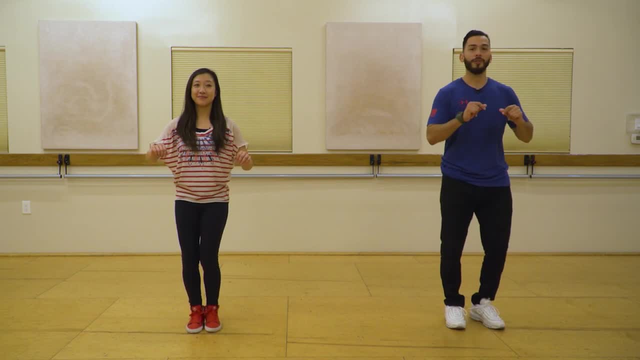 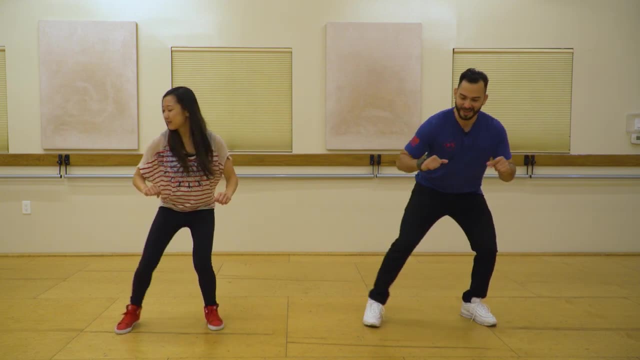 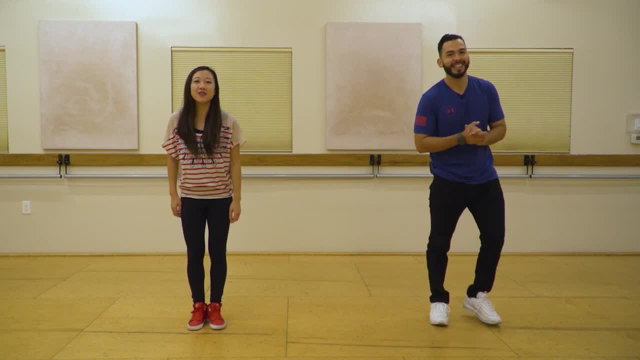 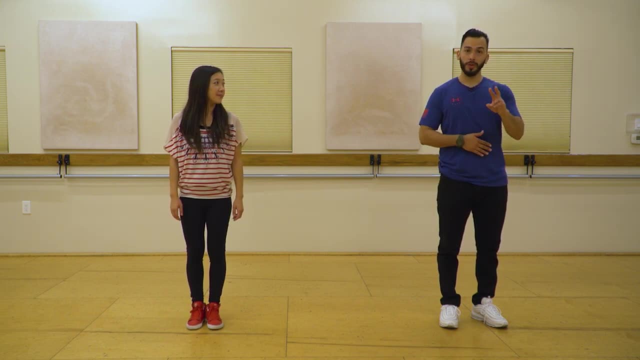 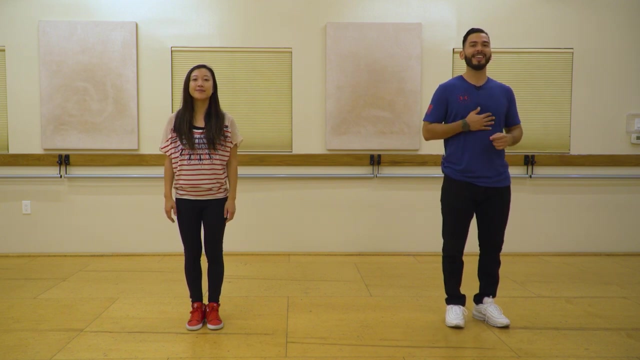 boom, boom, boom. Good, Nice, Shake all your worries off. Yes, We're going to shake it off, shake it off. So let's do this. We're going to do two up high and then we're going to do two down low. Sounds good, Ready. Five, six, five, six, seven, eight Left right. 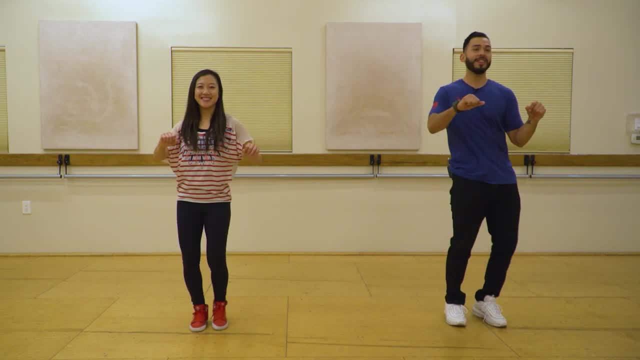 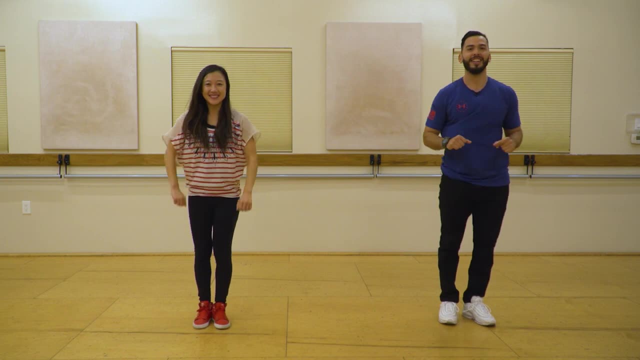 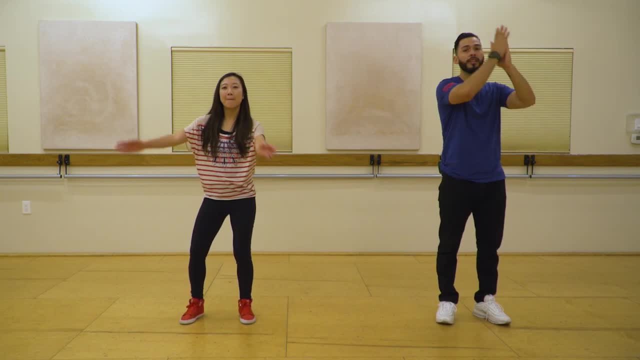 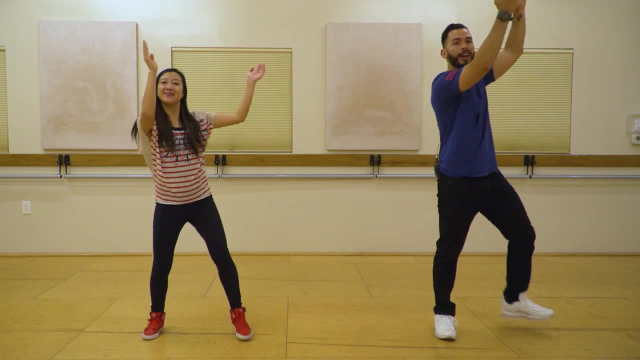 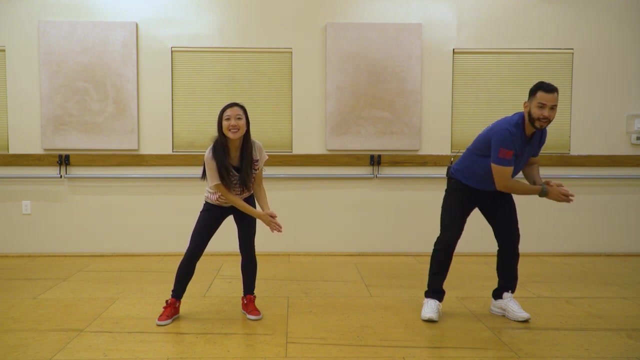 Now we're going to have some fun with it. We're going to clap, So we're going to start always to the left. We're going to clap here- Boom. We're going to step with the right- Boom. And then we're going to go low, Boom, boom. And then we go back to the left up there. 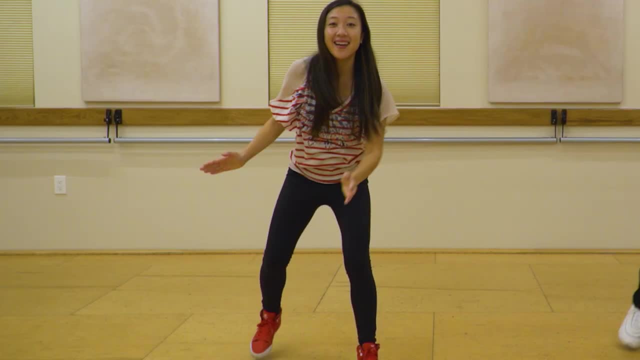 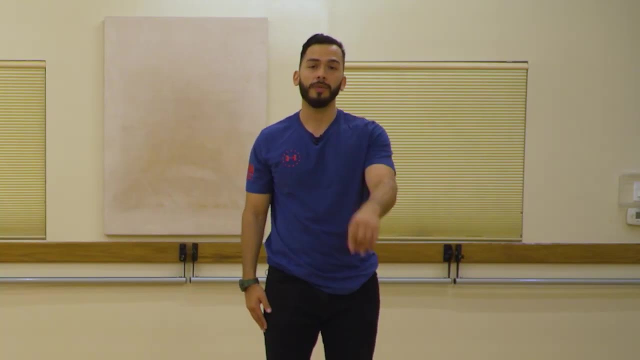 Ready And boom, Boom, boom, boom, boom. And then we stop in the center. So all together we're going to do it once Ready, Five, six, five, six, seven, eight, Boom, boom, boom, boom One. 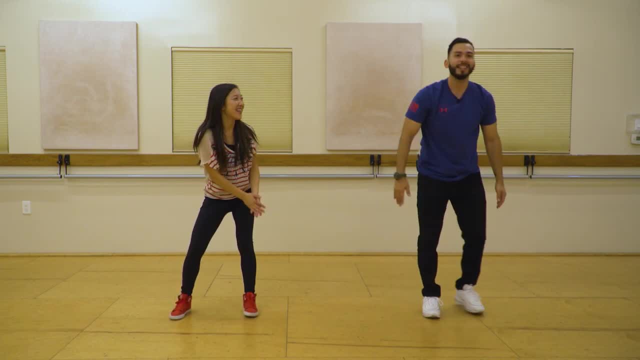 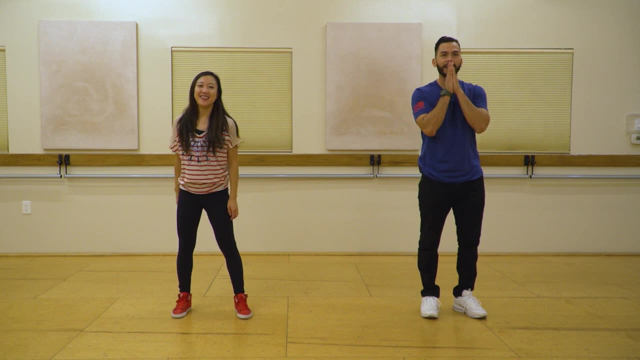 more time. Boom, boom, boom, boom And center. Hey, Nice, I want to try playing the drums. Oh yes, That's a good one, I like that one. So let's do this As soon as we hit. 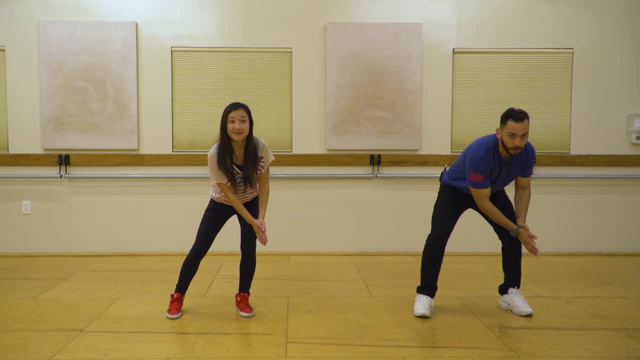 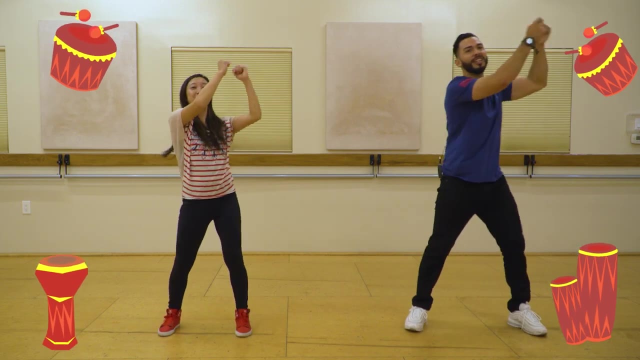 finish clapping. We're going to end it here right Now. we're just going to go into our drums: Ready Five, six, seven, eight And drums, drums and drums, drums, drums, drums and drums. Nice Now. 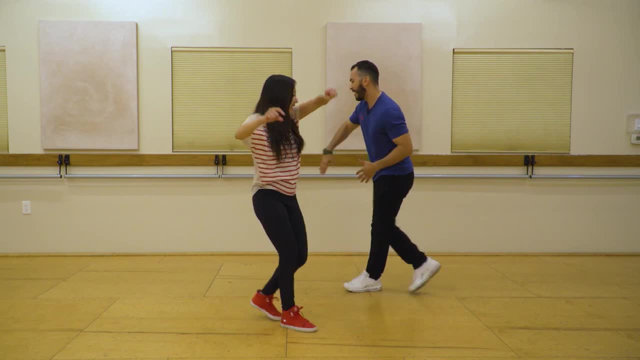 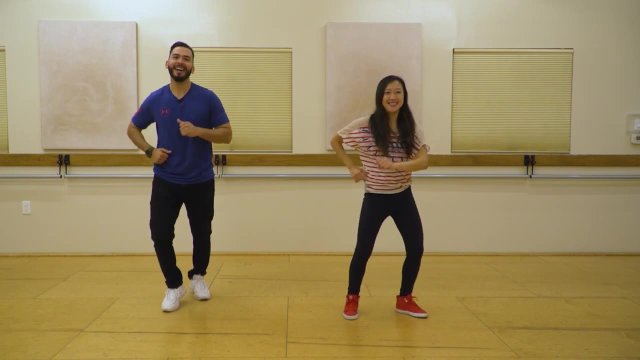 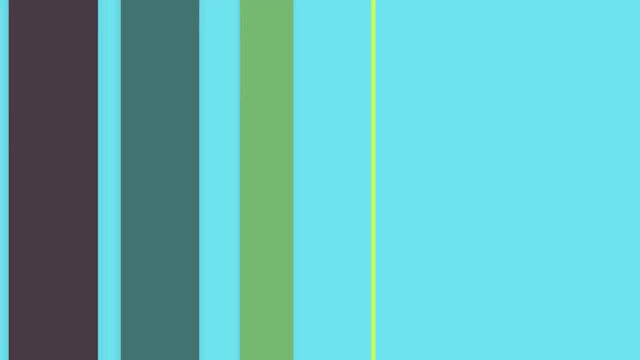 music. Yeah, Let's do it. Let's do it Ready. One, two, three, four, five, six, seven, eight. One, two, three, five, six, seven. One, two, three, five, six, seven. One, two, three, five, six, seven. One, two, three. 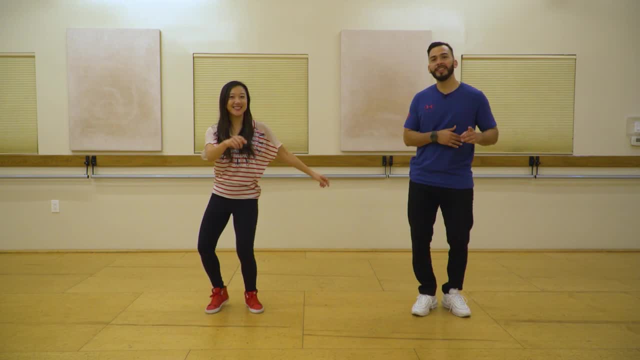 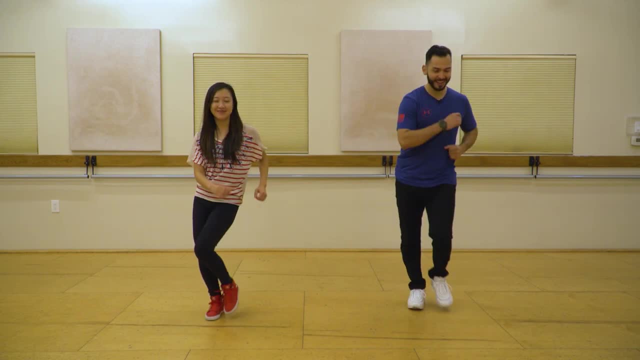 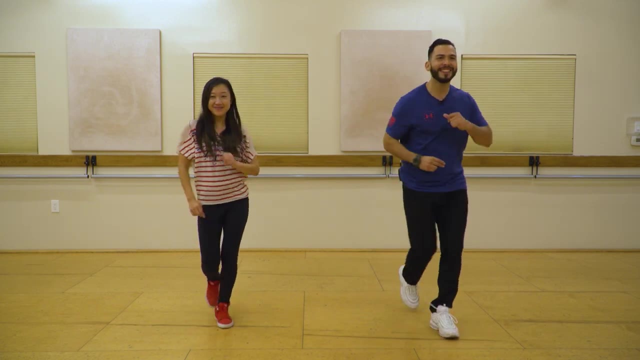 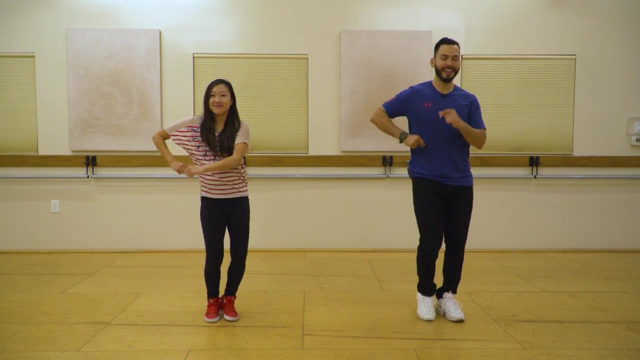 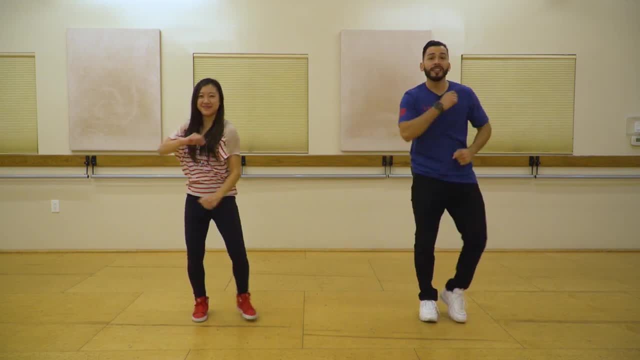 One, two, three to side. Ha hey, ha ha. boom, boom, Boom, boom, boom. Good job, keep it up 了. Let's do the cross. Let's do the cross continuously. boom, boom, Yes, boom. 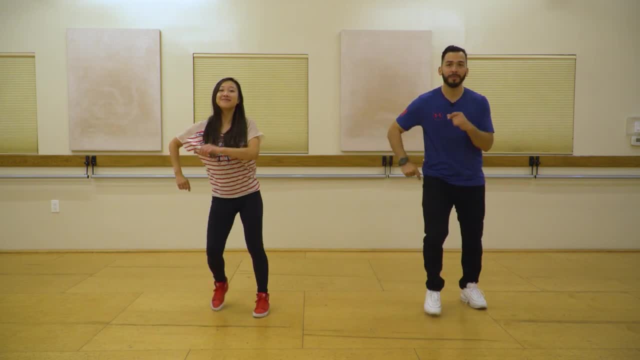 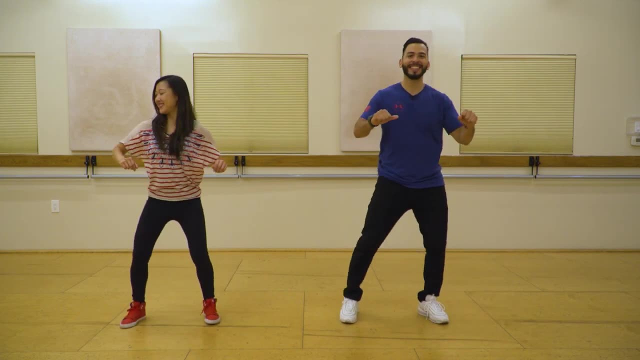 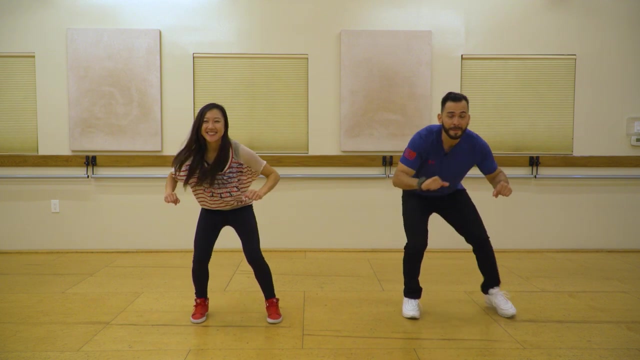 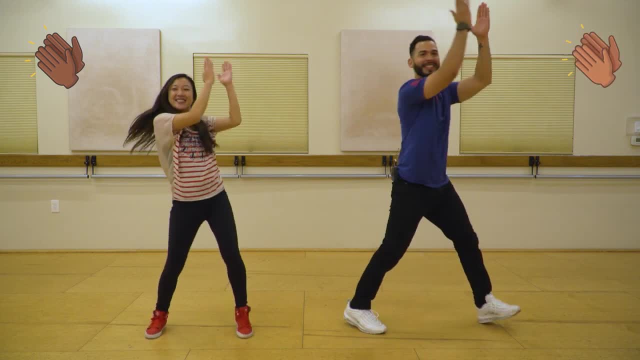 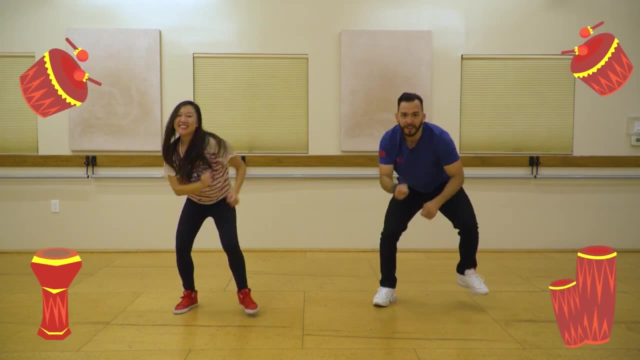 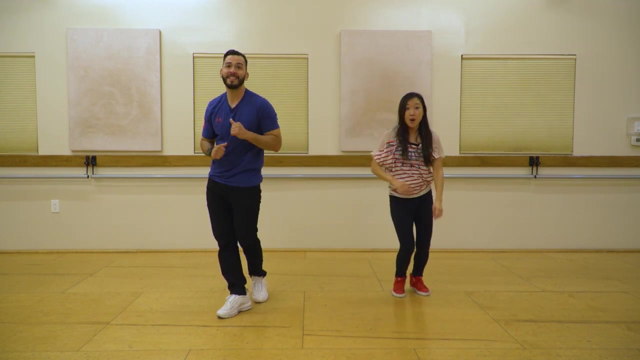 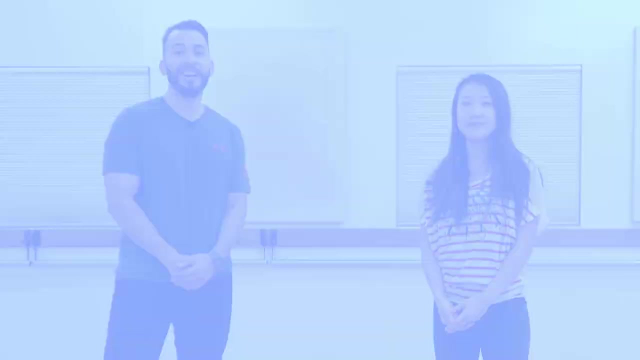 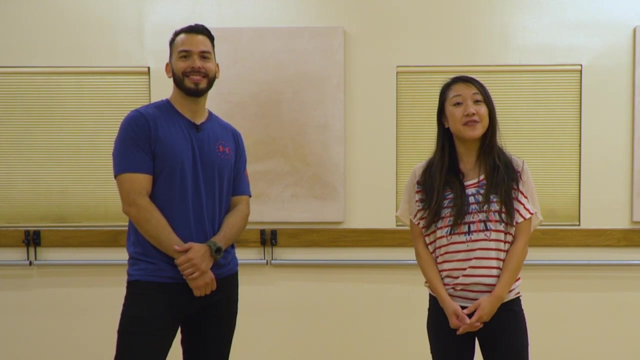 Where the drums at One, two, three, four, One, two. All right, how was that you guys? Did you have fun? I know I did. I did too. I hope you guys enjoyed our first salsa class. Thank you, Jesse, so much for teaching us. 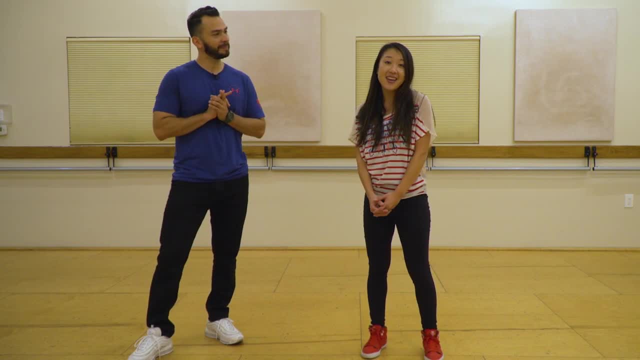 And don't forget you guys. if you have more classes you want to try, subscribe to CJ and Friends and we'll see you guys next time. Bye.